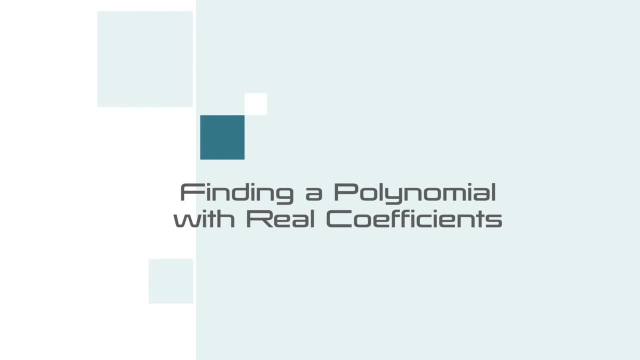 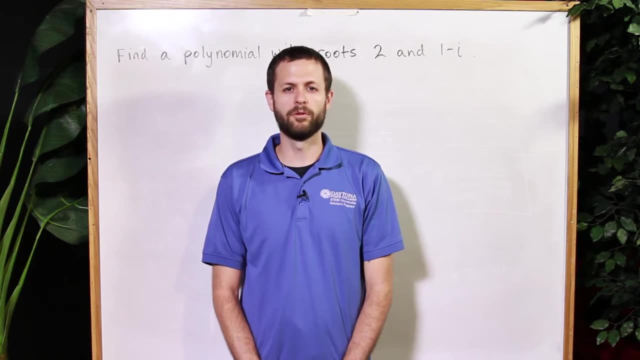 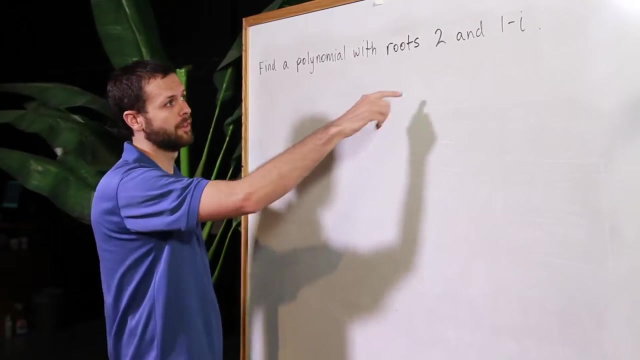 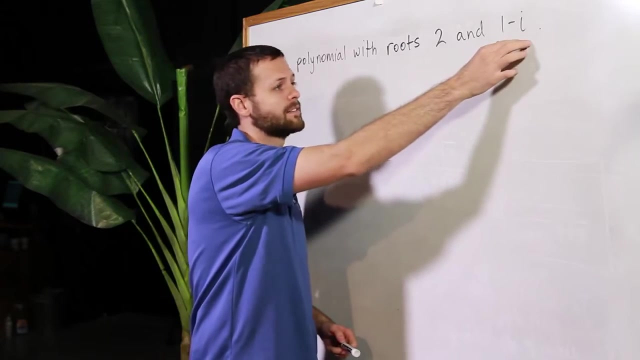 In this problem we're asked to find a polynomial with real coefficients given two of the roots. We don't know what the polynomial is, but we do know that the roots are 2 and 1 minus. i Remember that by the conjugate pairs theorem: if 1 minus i is a root, then 1 plus i must also be a root. 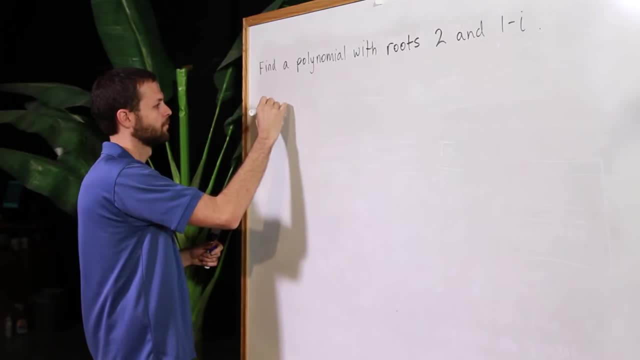 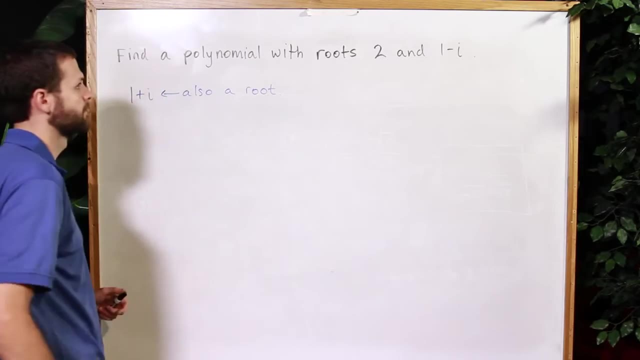 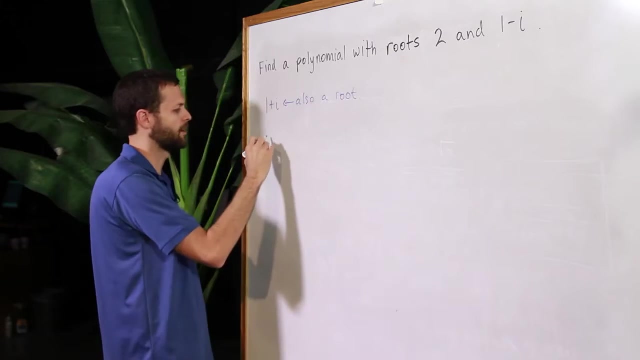 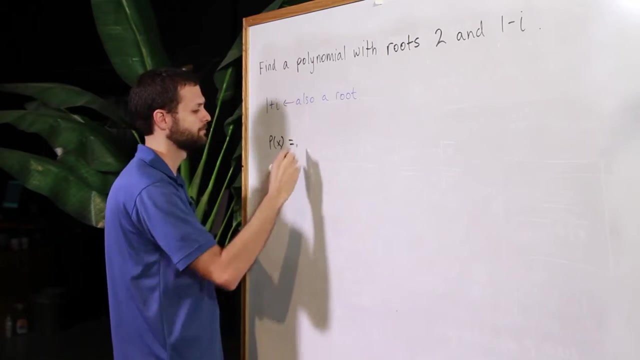 We're going to make a note of that. Since 2 is a root, I know that x minus 2 must be a factor. I'm going to call my new polynomial P. I can write this new polynomial as a product of the factors. 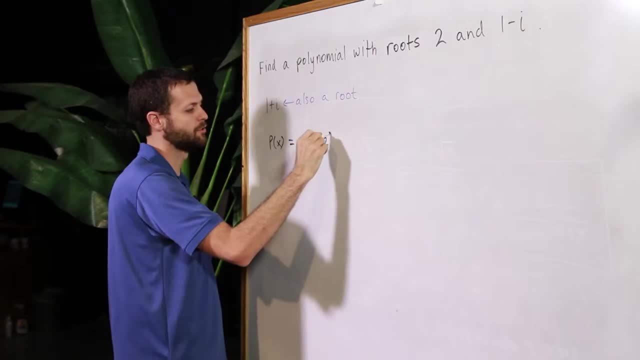 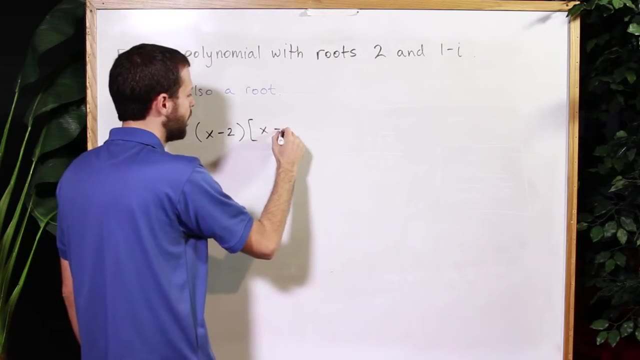 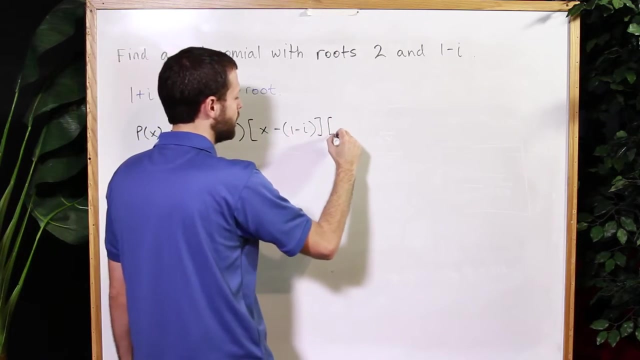 Like I said, since 2 is a root, I know that x minus 2 must be a factor. Since 1 minus i is a root, I know that x minus 1 minus i must be a factor. Since 1 plus i is a root, I know that x minus 1 plus i must be a factor. 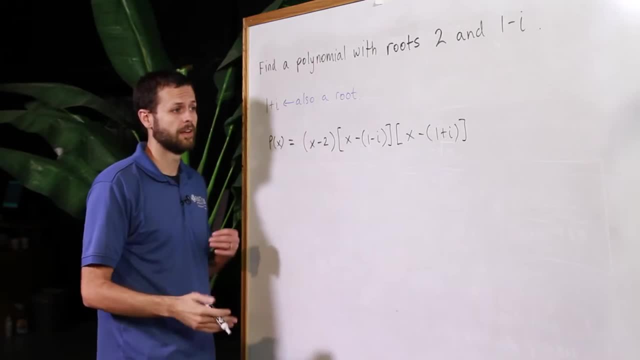 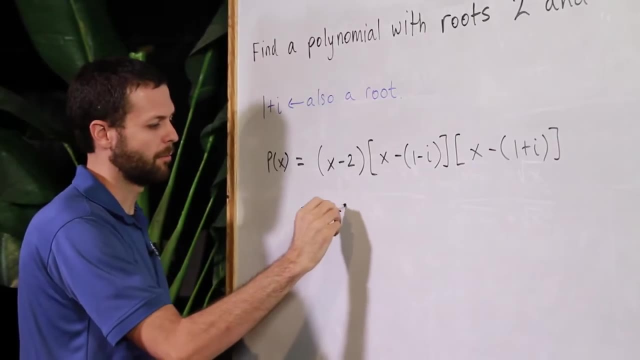 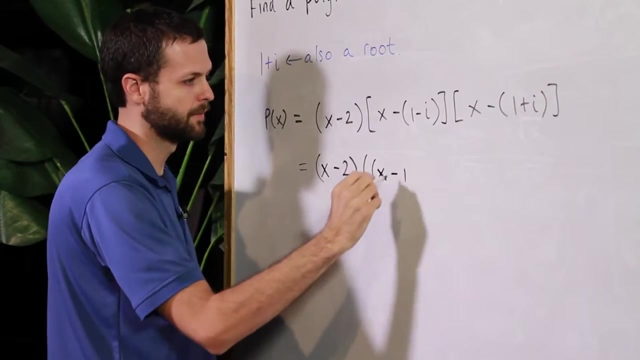 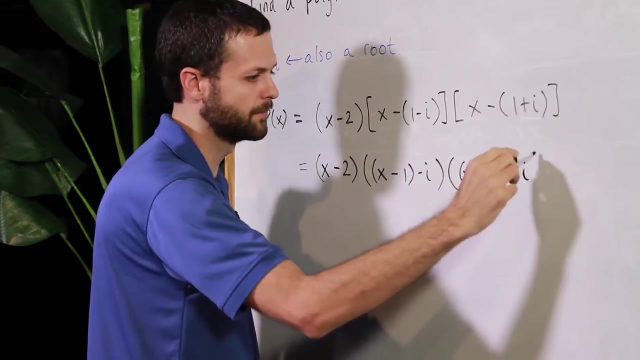 I can then proceed to multiply these out. If I'm creative and observant, I can multiply this fairly quickly. Upon rearranging this term and this term, I can write x minus 1 minus i Over here. I can write x minus 1 plus i. 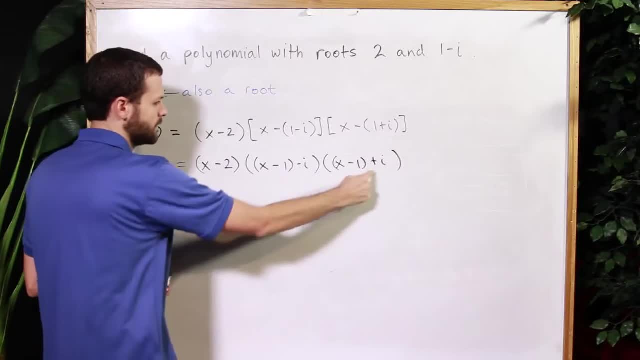 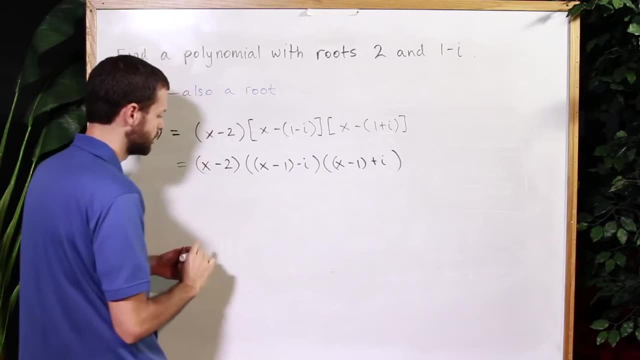 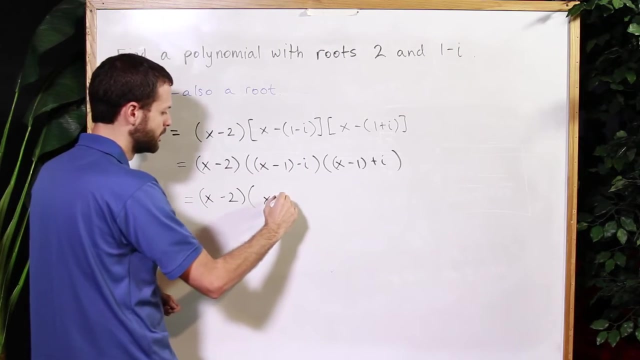 Remember that just looking at these last two expressions here, I can multiply these out, since these are conjugates to the following. I'm going to leave this x minus 2 alone for just a moment. This becomes x minus 1.. This becomes x minus 1, squared plus 1.. 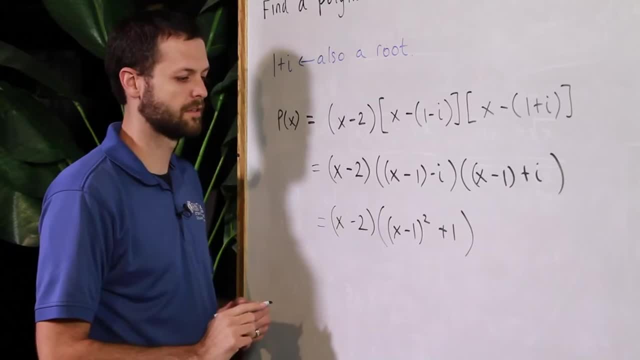 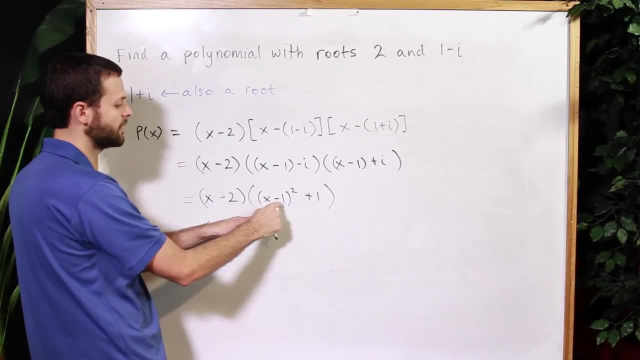 You can check this with FOIL, if you like, or by multiplying this out. in other words, We can keep going. I now have x minus 2.. Let's go ahead and expand this out. Remember that this is not x squared minus 1 squared. 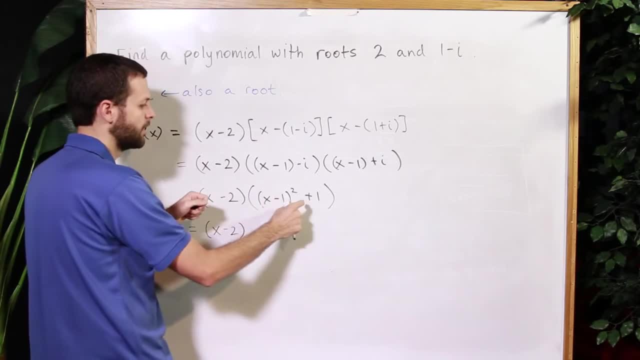 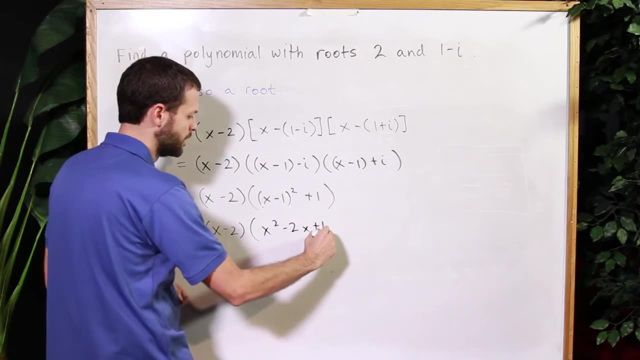 You need to expand this out. This is actually x minus 1 times x minus 1, or a perfect square trinomial: x squared minus 2x plus 1 plus 1.. This one comes from here. Let's simplify in here before we continue. 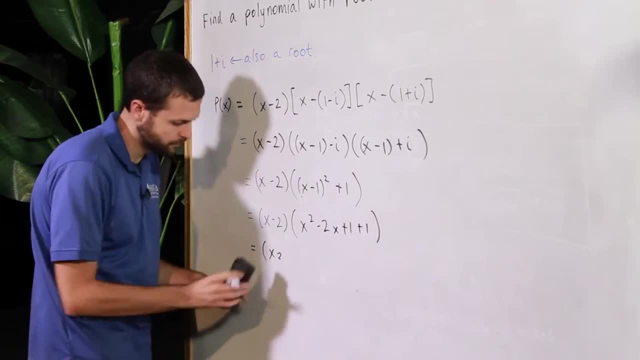 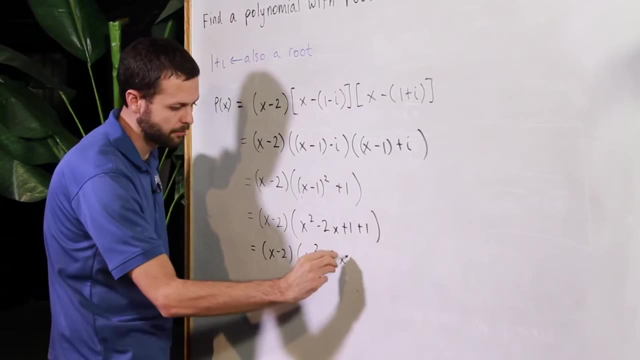 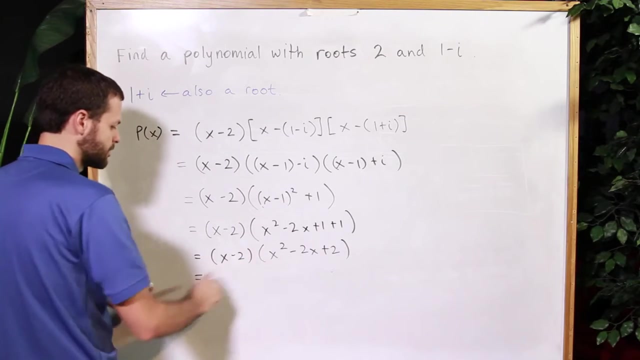 This becomes x minus 2 times x, squared minus 2x plus 2.. Again, let's multiply this out. I now have x times x squared. That's just x cubed x times minus 2x, minus 2x squared. 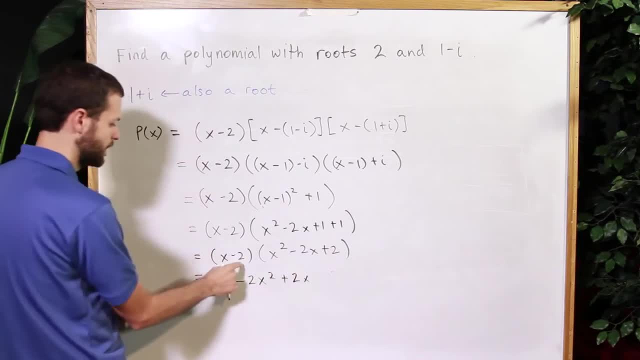 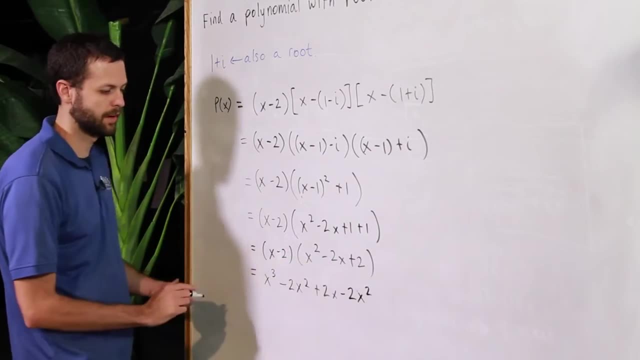 x times 2.. That's plus 2x. Do it again for minus 2.. Minus 2 times x squared: That's minus 2x squared. Minus 2 times minus 2x, That's plus 4x. 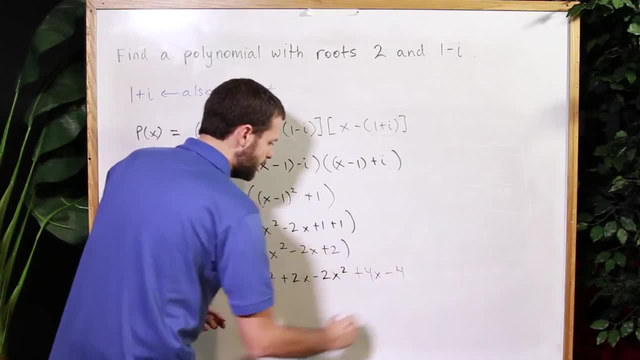 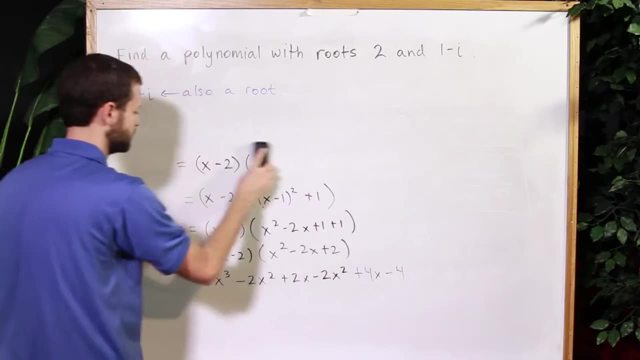 Minus 2 times 2. That's minus 4.. Now all I have to do is combine like terms. Let me just make a little bit of room. I'll look up here. This is what we have. I can now write my polynomial. 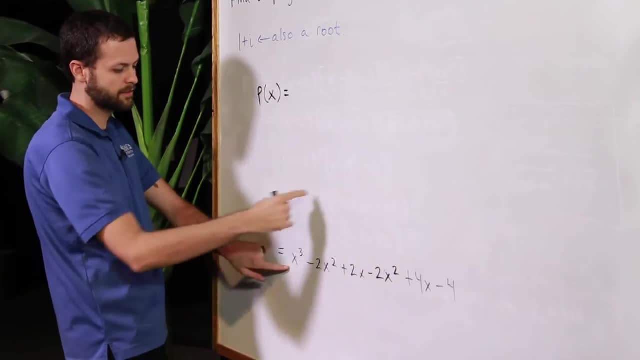 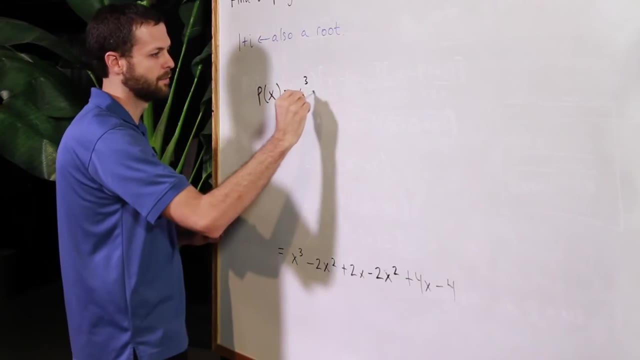 which I called p of x as follows: There's no other x cubed term, so I just have this x cubed by itself, Minus 2x squared. minus 2x squared, That gives me minus 4x squared. 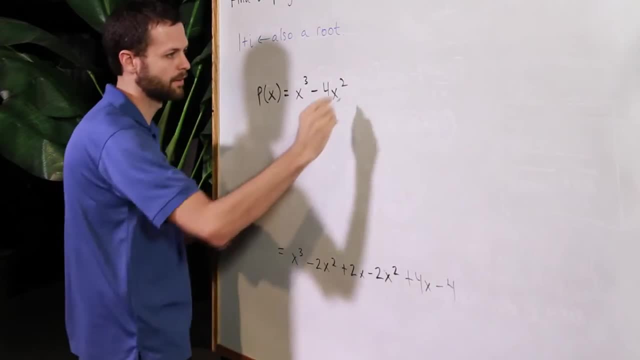 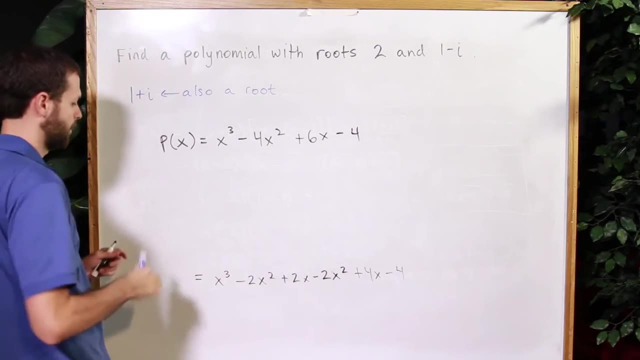 Then I have x terms, 2x and 4x. That gives me positive 6x. Then I finally have minus 4 left over. here I now have obtained a polynomial with real coefficients 1, minus 4,, 6, and minus 4,. 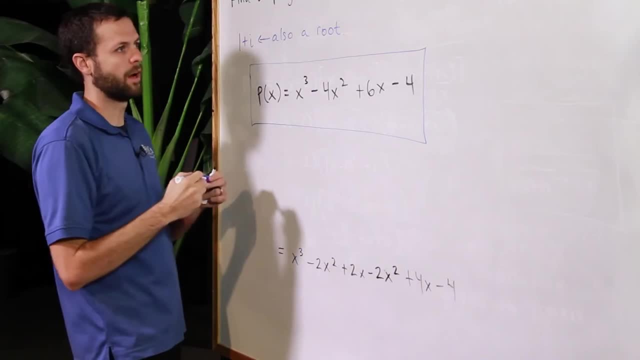 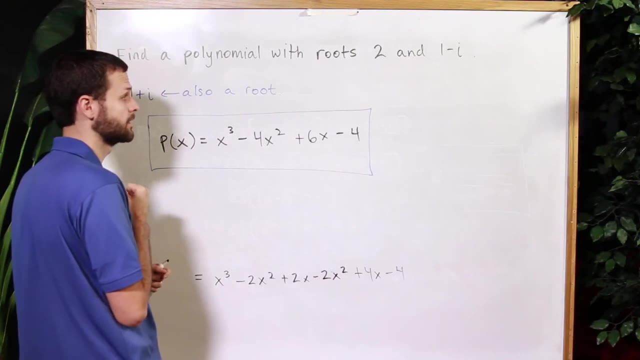 that has the roots 2, 1 minus i and 1 plus i. Again, what it means to have a root is that that's where this function, this polynomial, will cross the x-axis. Notice that two of them are complex numbers. 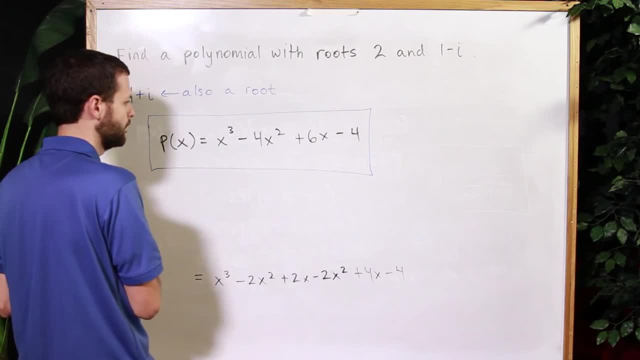 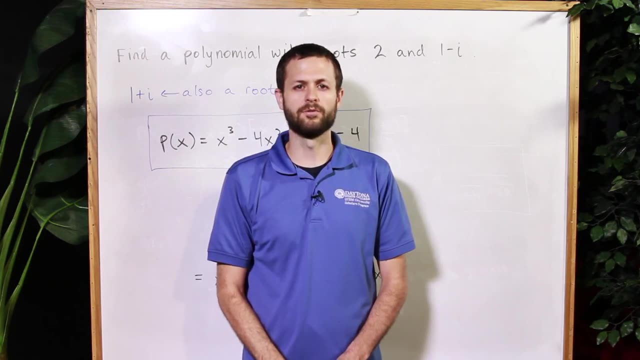 containing an imaginary component. In this problem, we use the complex conjugate pairs theorem in order to arrive at a polynomial that contains real coefficients only. Thank you for watching.